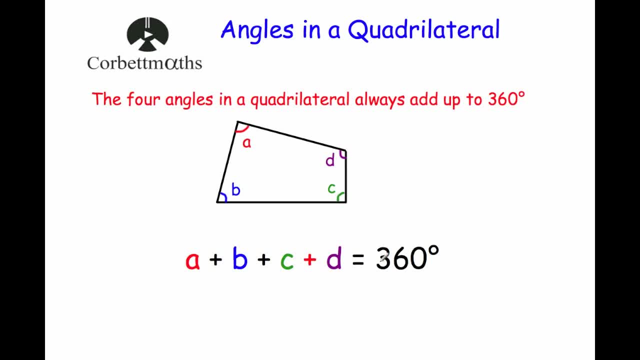 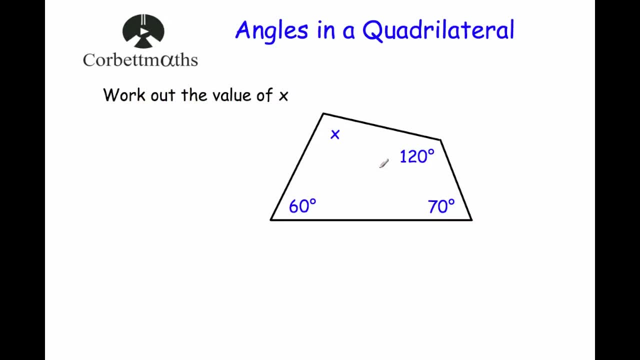 A plus B, plus C plus D would give you 360.. Okay, let's have a look at a typical question now. So here we've got a quadrilateral. It's got four angles and we know three of them. We know 60, 120 and 70.. We've been asked to find the size of this angle X. So 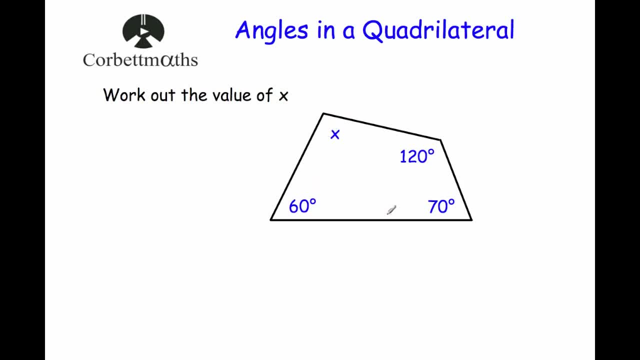 if you want to find a missing angle in a quadrilateral, you add up the ones that you know and take it away from 360.. So we're going to add up 120, 60 and 70.. We'll add those up, So 0 plus. 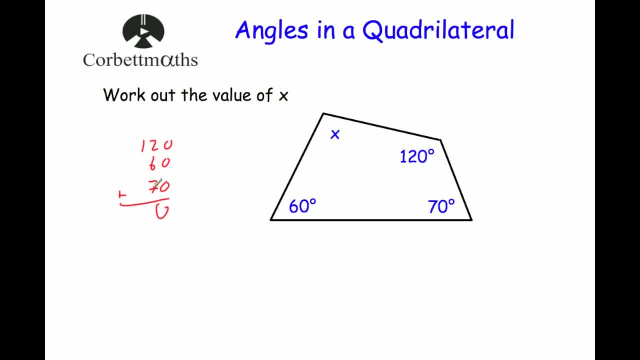 0 plus 0 is 0.. 2 plus 6 is 8 plus 7 is 15.. So put the 5 down and carry the 1.. And 1 plus 1 is 2.. So when you add up these three angles, we get: 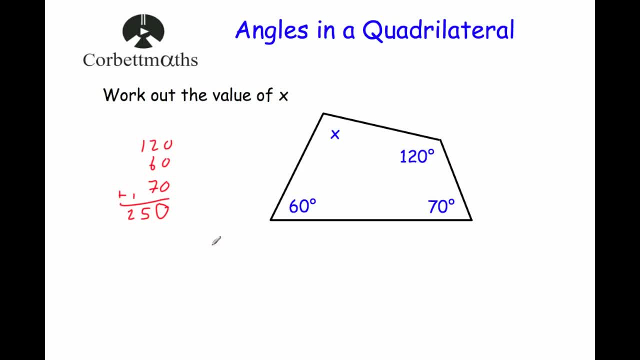 250.. Now we're going to take that away from 360.. So 360 minus 250. And when we do that we get 0. take away 0 is 0.. 6 take away 5 is 1.. And 3 take away 2 is 1.. So this angle X is: 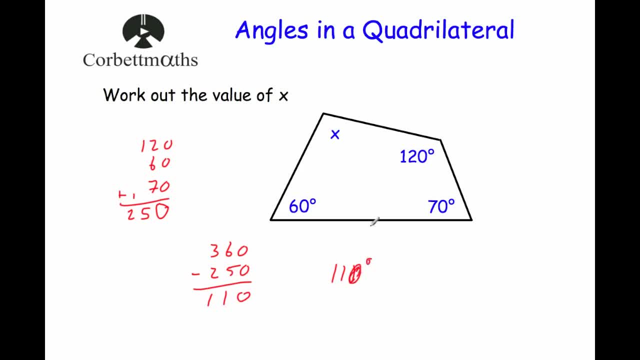 equal to 110 degrees, And that's it. So if you want to find a missing angle in a quadrilateral, if you know three of them, just add the three angles up and take it away from 360 degrees. Okay, now what we're going to do is we're going to look at some special angles, So we're 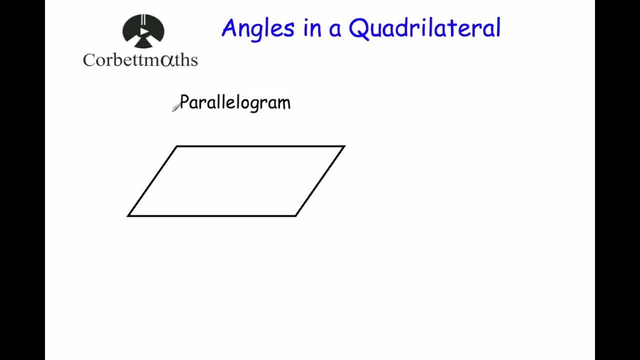 going to show quadrilaterals. So here we've got a parallelogram Now. in a parallelogram the opposite angles are equal to each other. So in other words, this angle, the obtuse one, is equal to the other obtuse angle there, And also the acute angles are equal to each. 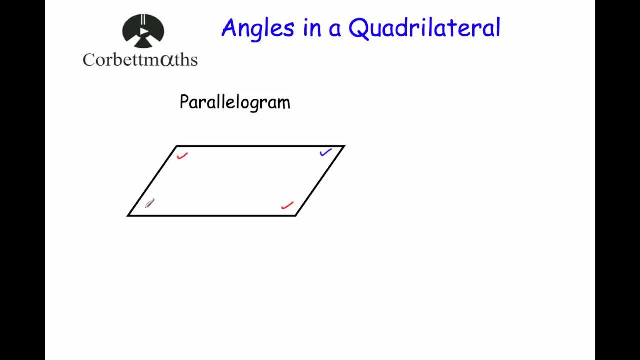 other. So this acute angle is equal to the opposite angle, which is also acute. So the opposite angles in a parallelogram are always equal to each other. So we have a look at a question now. Here we've got a parallelogram and we've been asked to find the sizes of 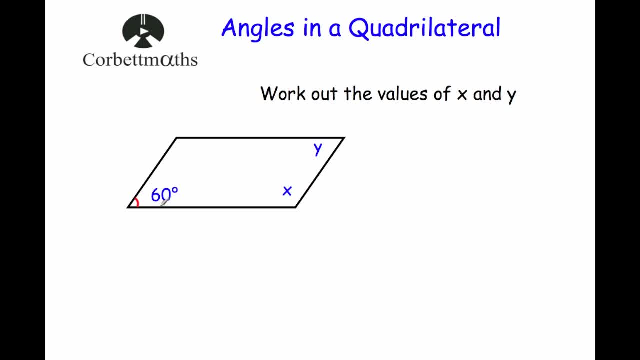 angle X and angle Y. So, first of all, we know that this angle is 60 degrees, So the opposite one, Y, will also be equal to 60 degrees, And if we want to find the size of angle X, what we're going? 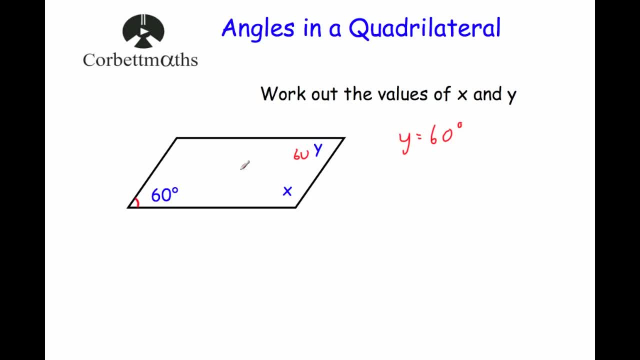 to do is we're going to add the two angles that we know, the two 60s together, And if we take that away from 360, we'll see what's left of the other two angles, And then, if we half it, we'll get what X is. So we're going to do 60 plus 60. So 60 plus 60 is equal. 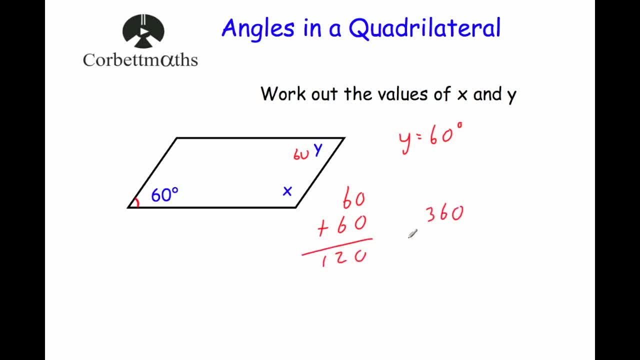 to 120.. And if we take that away from 360 degrees, that leaves us with 240.. So in other words, X and the opposite angle add together to be 240 degrees, And if we half that, so if we divide that by two, we're going to find the size of X. So two divided. 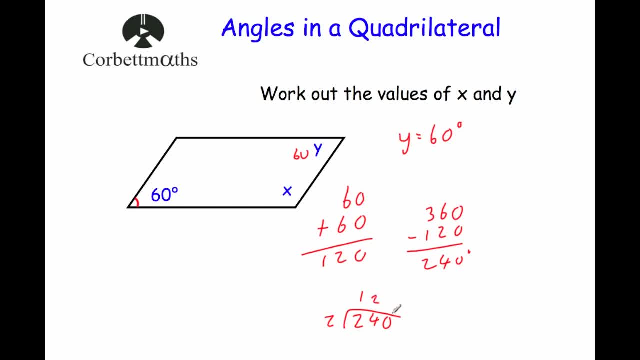 by two is one, Four divided by two is two, And zero divided by two is zero. So the angle X is equal to 120 degrees. Okay, our next quadrilateral, Our next special quadrilateral is a kite. A kite has got a. 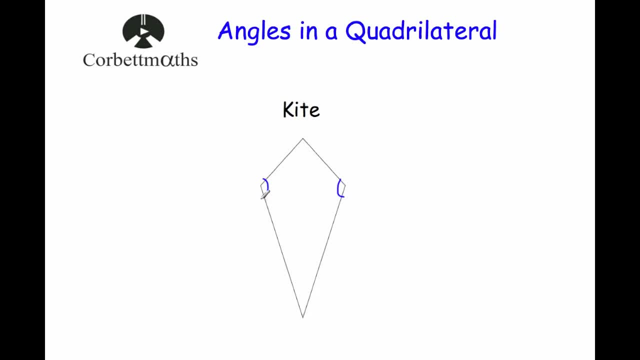 line of symmetry, vertically through the top and the bottom, like so. So it's got a line of symmetry. So the two opposite angles, the ones on the side, here and here, are equal to each other. So, for instance, if this was equal to 140 degrees, the opposite one here. 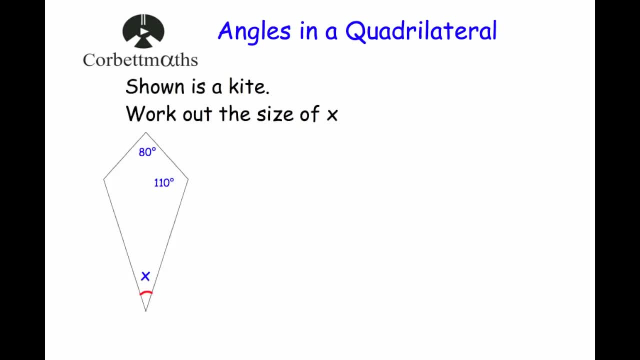 would also be equal to 140 degrees. So here's a typical question. It says: here's the kite, Work out the size of angle X. So here we've got the kite, We've got the top angle's 80,, the one on the right's 110, the one on the bottom's X, and this one's missing Now because 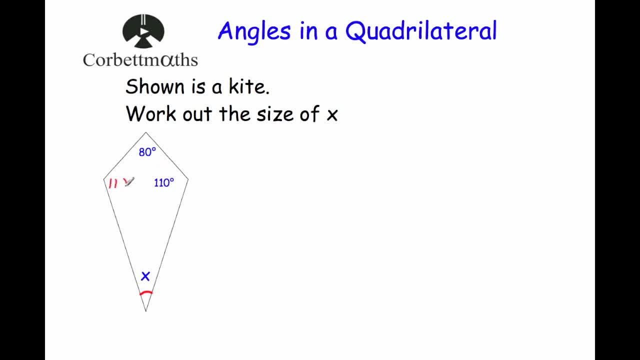 it's a kite and it's got a line of symmetry. this one will have to be 110 degrees also. So we'll just add these three angles up together, So 110 plus 110 plus 80. And we'll see what we get. So zero one plus one plus eight is 10.. So put the zero down, kite the one, and 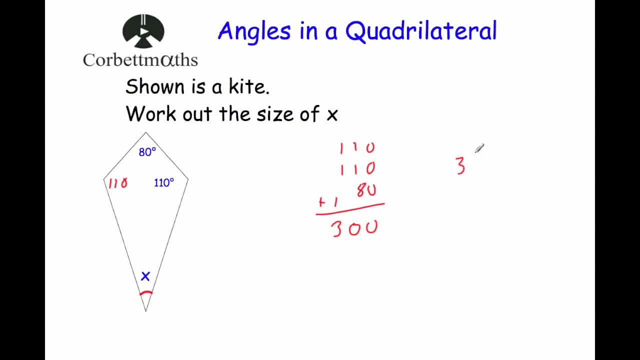 three. So these three angles add up to 300 degrees And if we take that away from 360, we see that 60 degrees is left. So the angle X is equal to 60 degrees. Okay, And our last special shape we're going to look at in this video is a rhombus, And a rhombus is just. 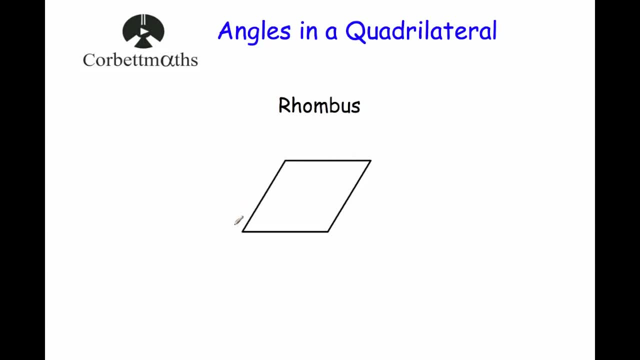 like a parallelogram, Um apart from, obviously, the sides are all the same length, but the opposite angles are the same also. So this angle, here the obtuse one, is the same as the opposite obtuse one, And the acute one here is the same as this acute one here. Okay, So the question says: